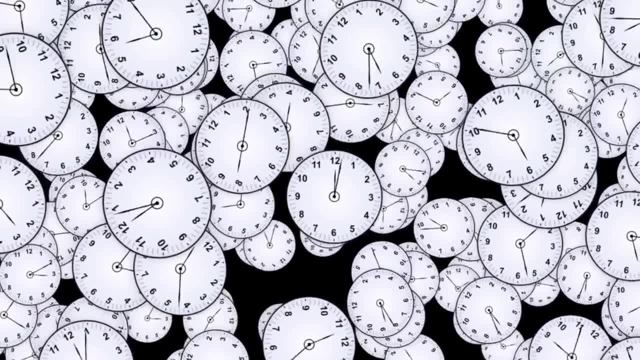 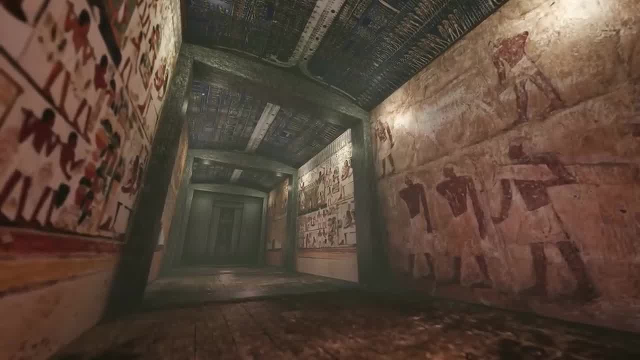 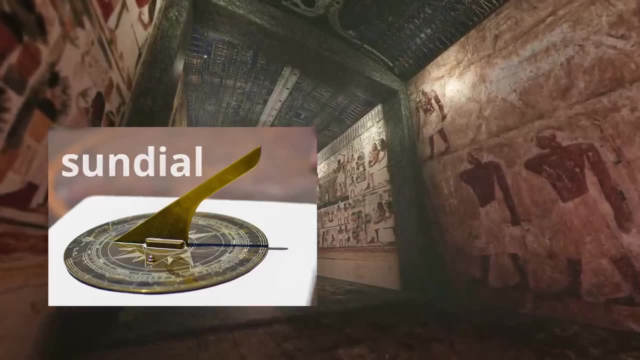 Clocks are amazing, wonderful inventions. Humans have used clocks for a really long time. In the ancient world, a common type of clock was the sundial. That's right, the sundial. Sundials are very accurate, but are not used often today. Have you ever asked what time it is? and 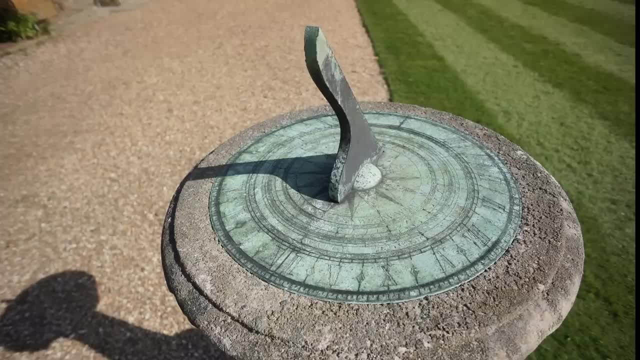 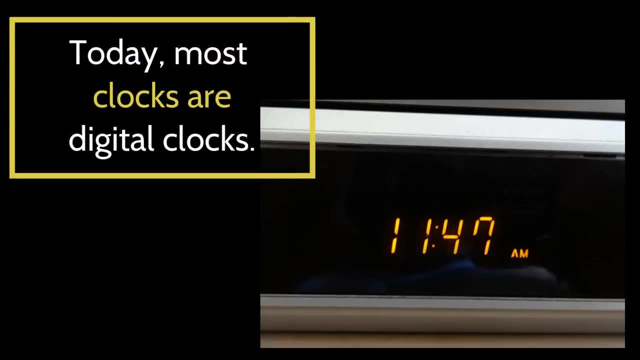 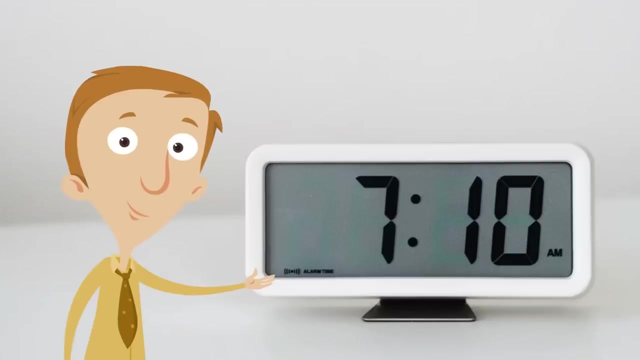 someone checks their sundial. Yeah, that isn't real common. Today most clocks are digital clocks. Digital clocks are really simple to use. They simply show the digits for the hour and minutes. So here we have a digital clock. Here on the left we see the hour. It is seven. On the 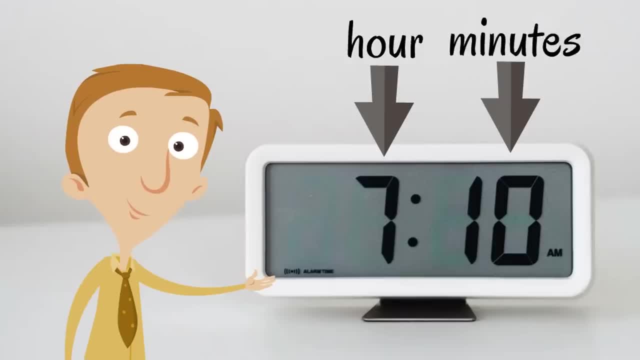 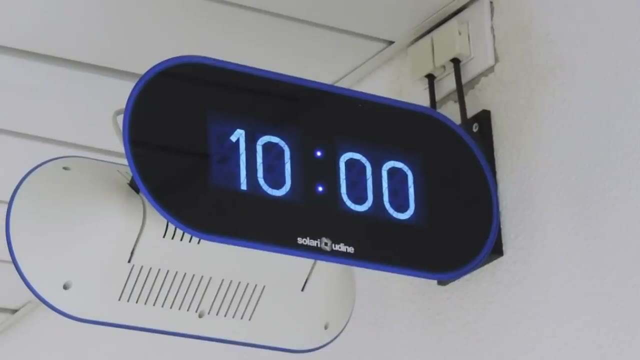 right, we see the minutes ten. So what time is it according to this clock? Yeah, it is 7.10.. Ten minutes past seven o'clock. What about this clock? Here is another digital clock. What time is it according to this clock? Yes, it is ten o'clock. On the left, we see the 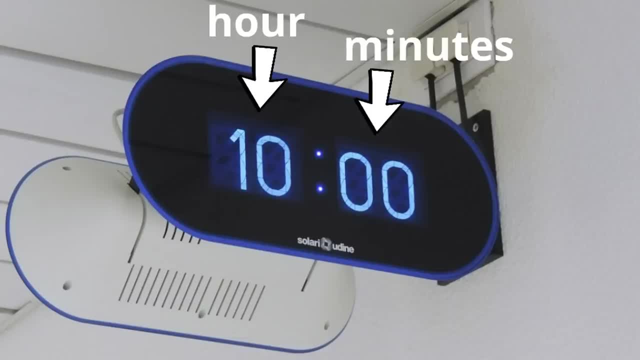 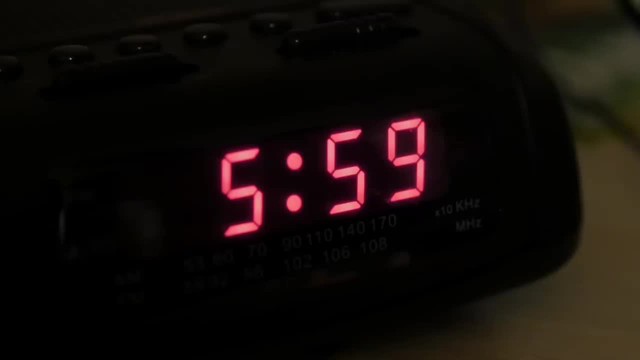 hour, which is ten, And on the right we see the minutes, which are just zeros, So it is exactly ten o'clock Now. digital clocks are not the only way we can use them. They are not the only way we can use them. They are the only way we can use them. They are the only way we can use them. 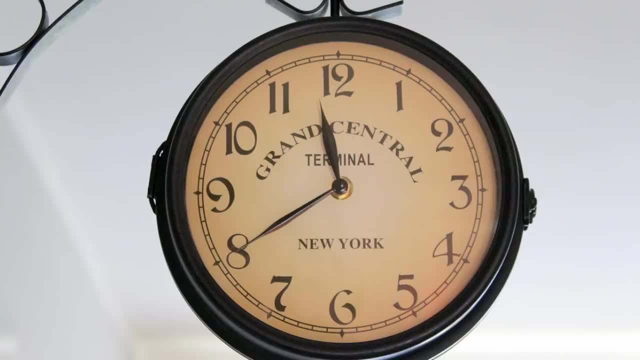 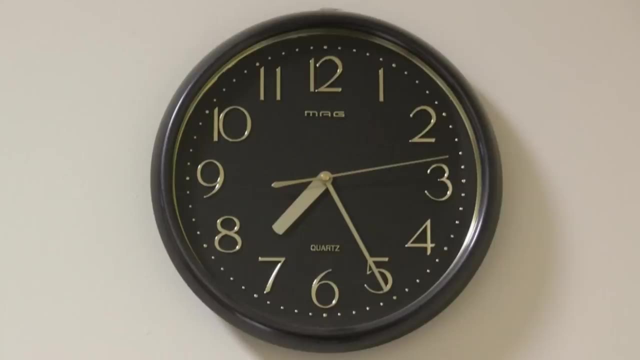 We can see what time it is. Have you ever seen a clock like this before? Yeah, This is called an analog clock. It is a different way to display time. In this video, we are going to learn how to read analog clocks, which will be super awesome because 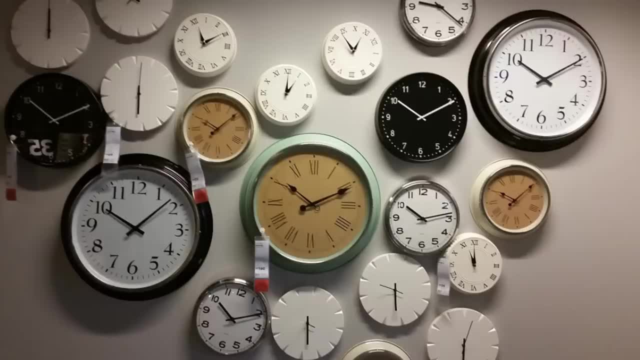 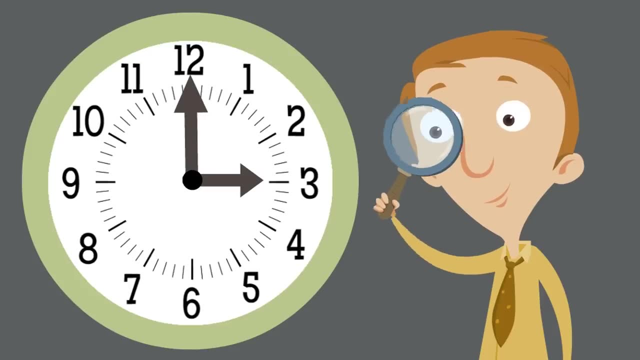 there are analog clocks all around us that want to be read. They want to show us the time. So, to start, we are going to learn some fun things. We are going to learn some fun things about the analog clock. The front is called the face of the. 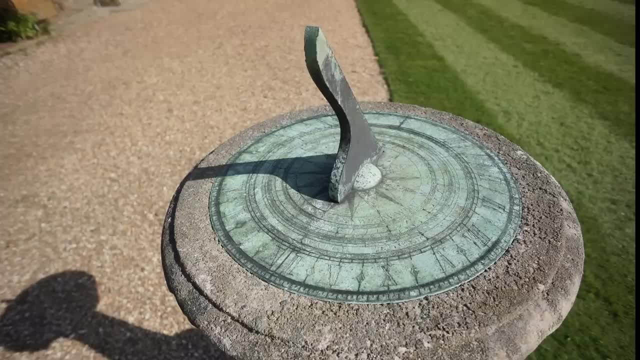 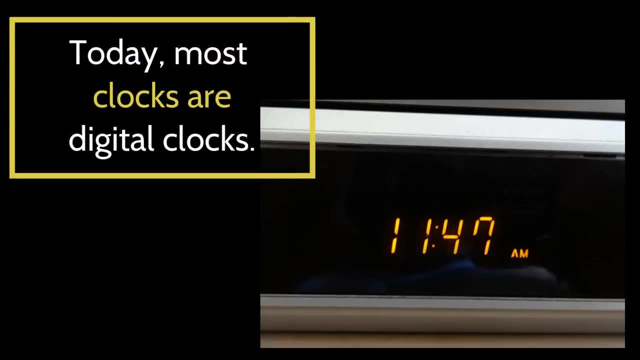 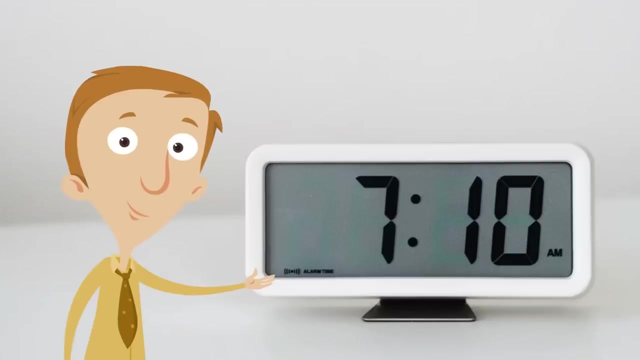 someone checks their sundial. Yeah, that isn't real common. Today most clocks are digital clocks. Digital clocks are really simple to use. They simply show the digits for the hour and minutes. So here we have a digital clock. Here on the left we see the hour. It is seven. On the 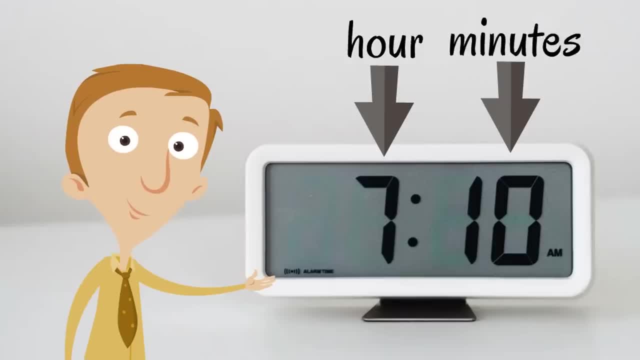 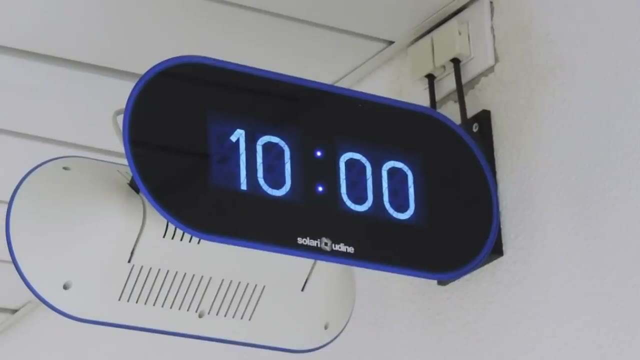 right, we see the minutes ten. So what time is it according to this clock? Yeah, it is 7.10.. Ten minutes past seven o'clock. What about this clock? Here is another digital clock. What time is it according to this clock? Yes, it is ten o'clock. On the left, we see the 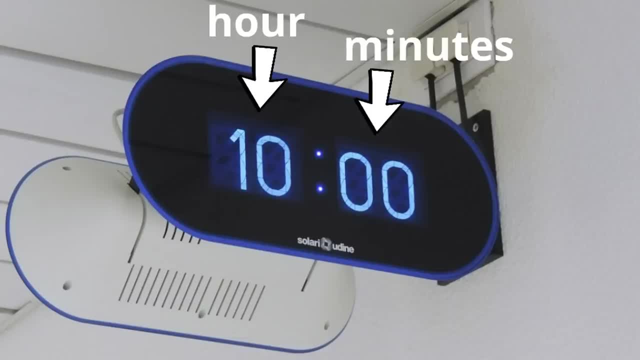 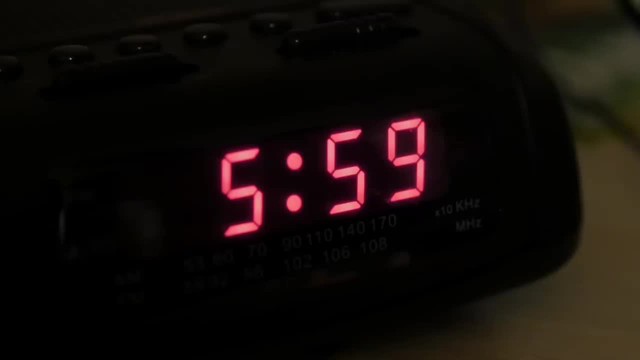 hour, which is ten, And on the right we see the minutes, which are just zeros, So it is exactly ten o'clock Now. digital clocks are not the only way we can use them. They are not the only way we can use them. They are the only way we can use them. They are the only way we can use them. 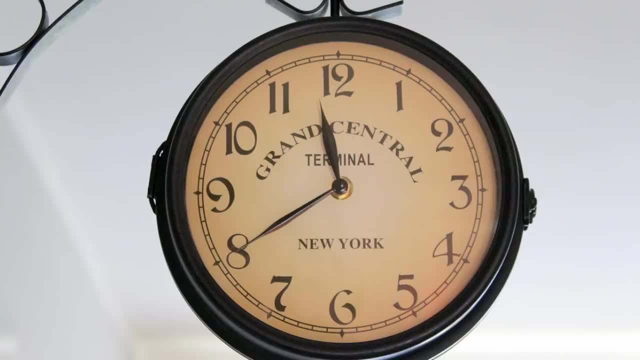 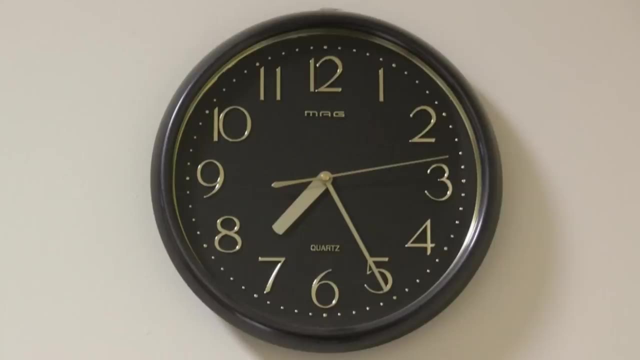 We can see what time it is. Have you ever seen a clock like this before? Yeah, This is called an analog clock. It is a different way to display time. In this video, we are going to learn how to read analog clocks, which will be super awesome because 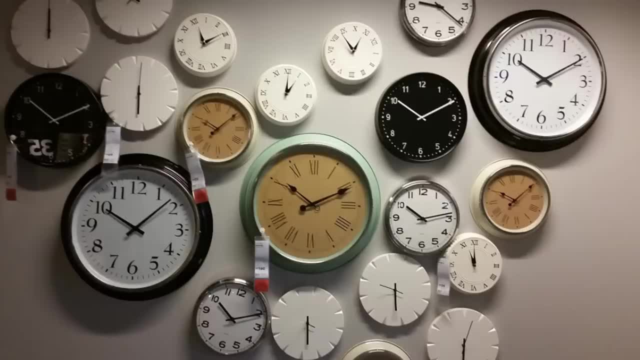 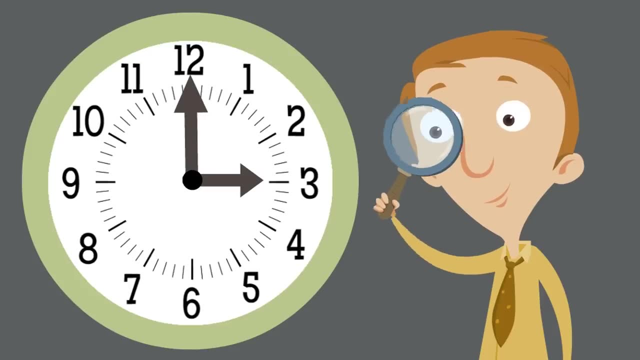 there are analog clocks all around us that want to be read. They want to show us the time. So, to start, we are going to learn some fun things. We are going to learn some fun things about the analog clock. The front is called the face of the. 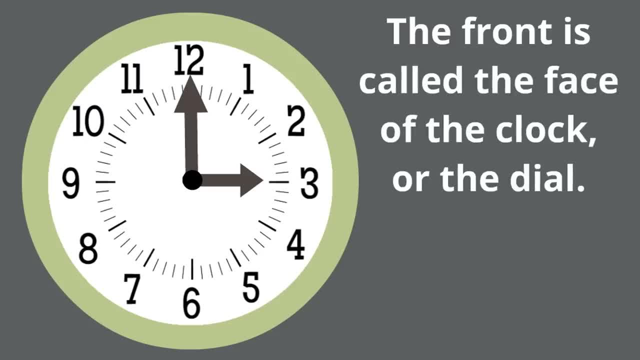 clock or the dial. Just like you have a face, an analog clock has a face. That's right. The face includes the numbers, the parts that spin and all the markings on the clock. The face, sometimes called the dial, has two main parts that point to the numbers and spin around. They are called hands. 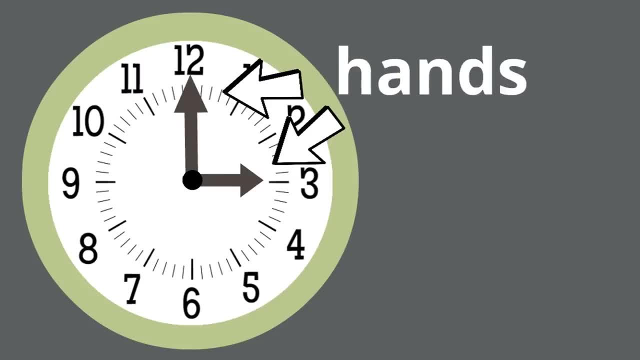 Isn't that interesting. The shorter hand is the hour hand. It shows us what hour it is. The hour hand is short. The longer hand is the minute hand. It points to the minutes. It's silly: Even though an hour is longer than a minute, the hour hand is. 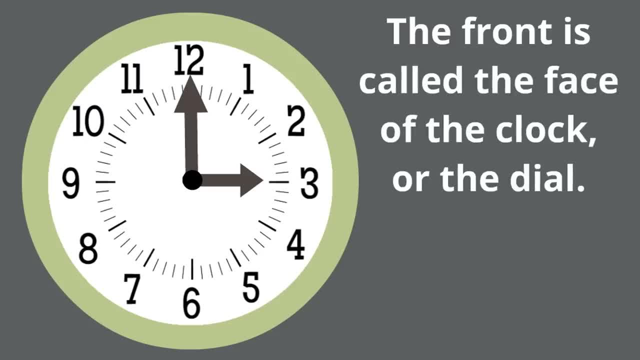 clock or the dial. Just like you have a face, an analog clock has a face. That's right. The face includes the numbers, the parts that spin and all the markings on the clock. The face, sometimes called the dial, has two main parts that point to the numbers and spin around. They are called hands. 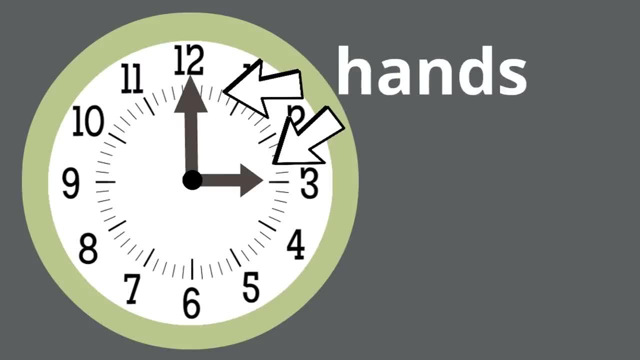 Isn't that interesting. The shorter hand is the hour hand. It shows us what hour it is. The hour hand is short. The longer hand is the minute hand. It points to the minutes. It's silly: Even though an hour is longer than a minute, the hour hand is. 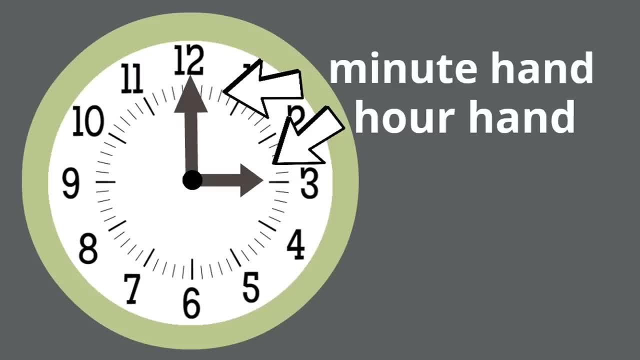 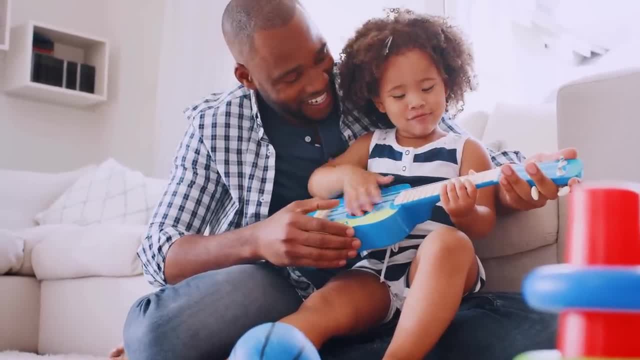 shorter. The hour hand is the short hand and the minute hand is the long hand. So, just like you, analog clocks have a face and usually have two hands. The short hand points to the hour, The long hand points to the minute, The minute hand points to the hour, The hour hand points to the 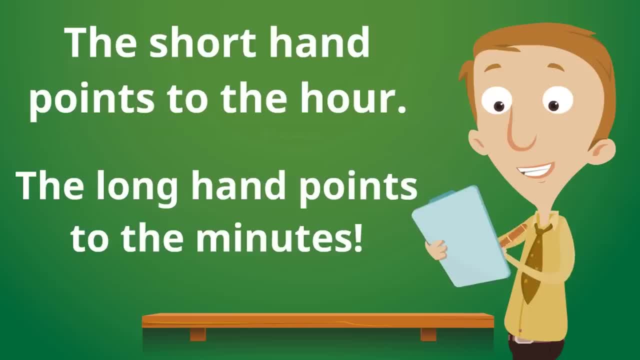 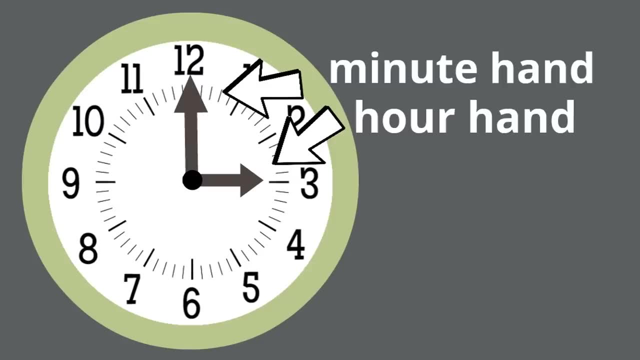 to the minutes. Let's go back to our analog clock and see if we can figure out what time it is showing, Just like we do with the digital clock. let's look at the hour hand, the shorthand, first. What number is it pointing at? Yes, at the number three. Great. So it is the. 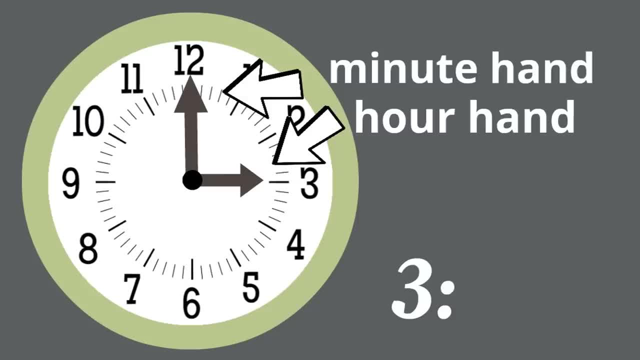 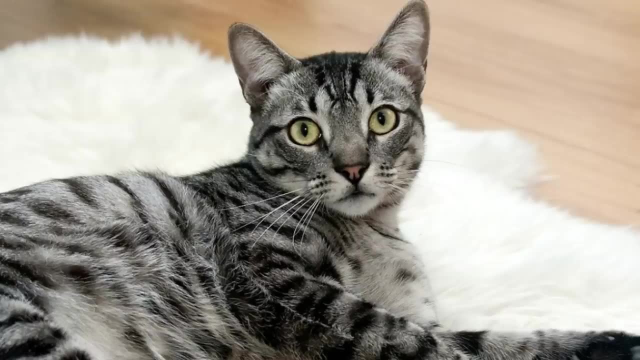 third hour. It is three something. Now we just have to read the minutes. The minute hand is the long hand, But how do we read the minutes? It only goes up to 12 and those big numbers are what we use for the hours. What do we do? Mr Whiskers, we're recording What. You know how to read the. 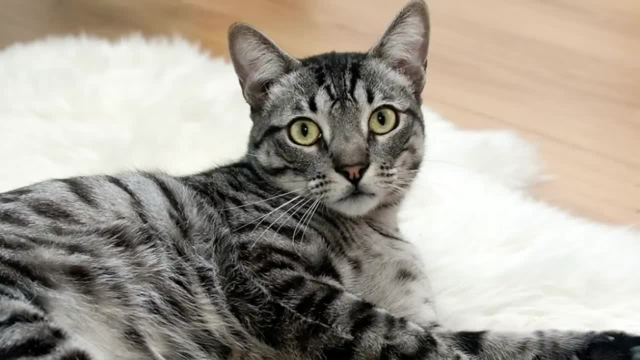 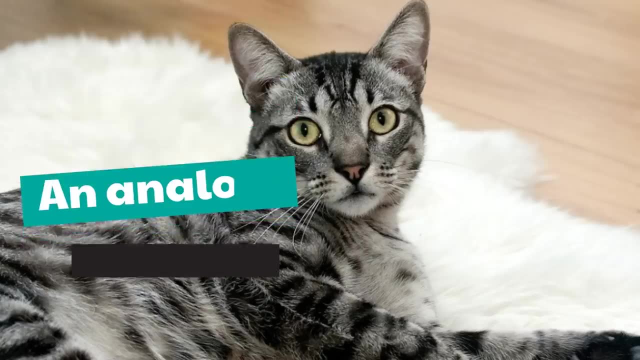 minutes on an analog clock. I didn't even know you knew how to tell time. You're a cat, You have a trick. Well, we should hear the trick. It's important for us to know how to tell time. Learn how to do this, Okay. An analog trick with Mr Whiskers. Okay, That's a little crazy. 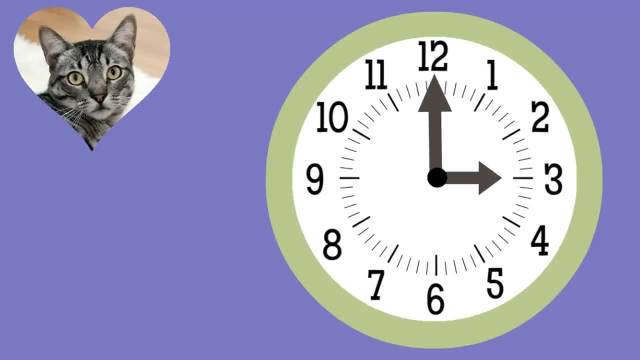 but that's okay, All right. So what's the trick? Oh, okay, So we need to count by fives to find out the minutes. That's a wonderful trick. That's amazing. You see all of those little lines in. 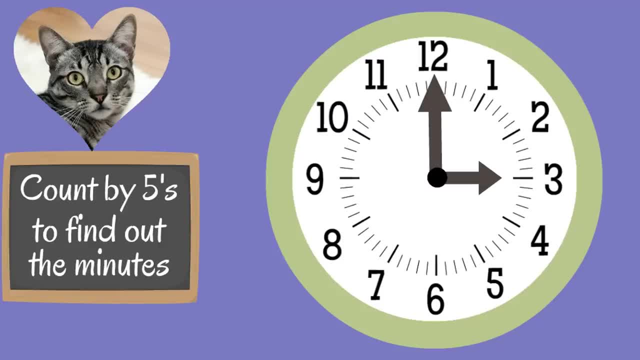 between the numbers on the face of the clock represent one minute. To find out the minutes we just have to count by fives around the clock Starting at the 12.. The 12 is like the starting line When the minute hand is at the 12,. 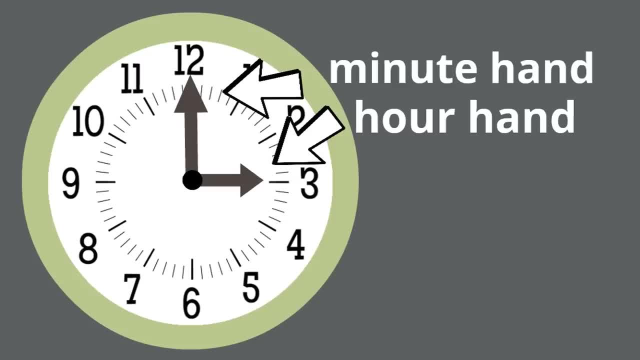 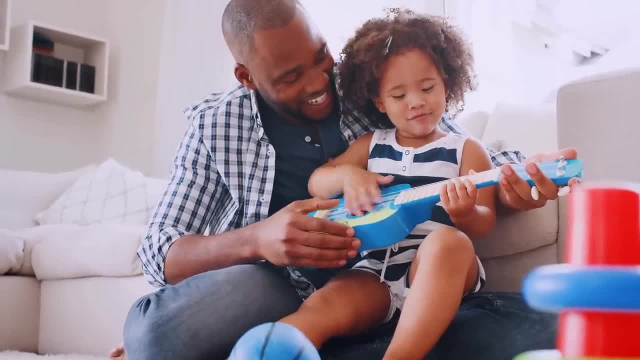 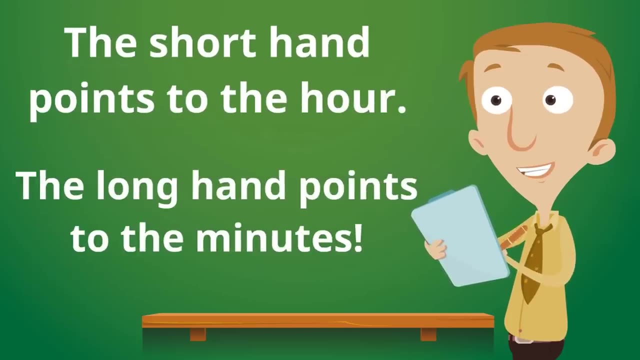 shorter. The hour hand is the short hand And the minute hand is the long hand. So, just like you, analog clocks have a face and usually have two hands. The short hand points to the hour, The long hand points to the minutes. let's go back to our analog clock and see if we can figure. 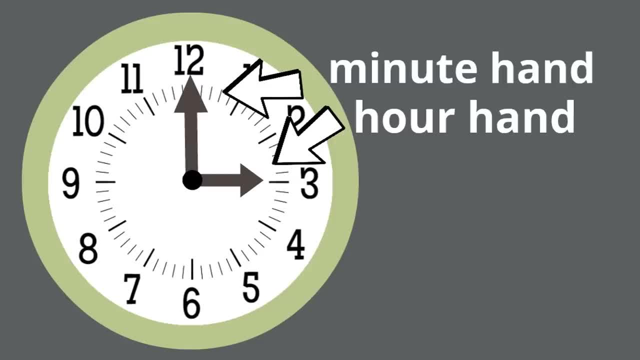 out what time it is showing, just like we do with the digital clock. let's look at the hour hand, the shorthand, first. what number is it pointing at? yes, at the number three. great, so it is the third hour. it is three something. now we just have to read the minutes. the minute hand is the long hand, but how do we read the? 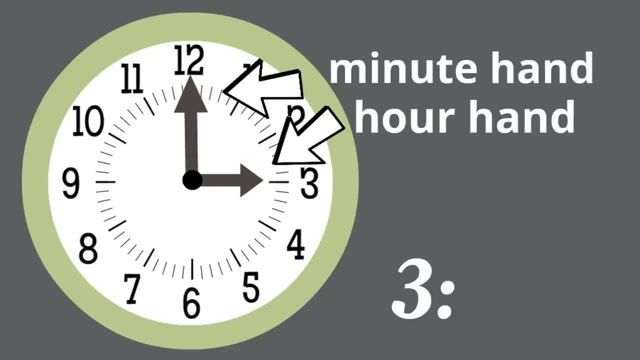 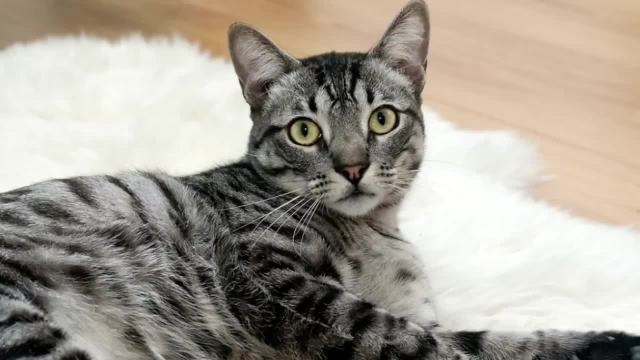 minutes. it only goes up to 12 and those big numbers are what we use for the hours. what do we do, mr whiskers? we're recording what. you know how to read the minutes on an analog clock? I didn't even know. you knew how to tell time. you're a. 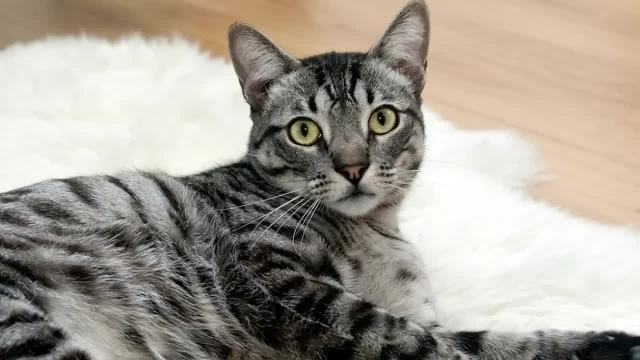 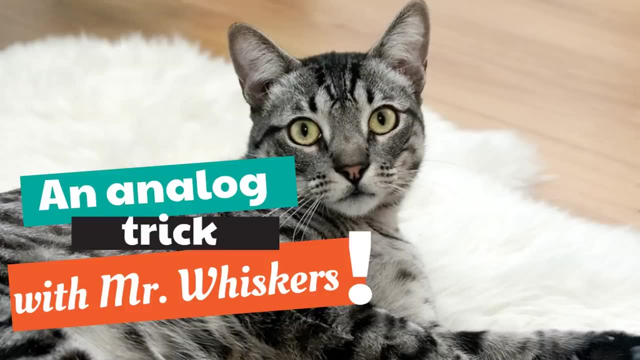 cat, you have a trick? well, we should hear the trick. it's important for us to learn how to do this. okay, an analog trick: well, we should hear the trick. it's important for us to learn how to do this. okay, an analog trick: we with mr whiskers. okay, this is a little crazy, but that's okay, all right. so what's? 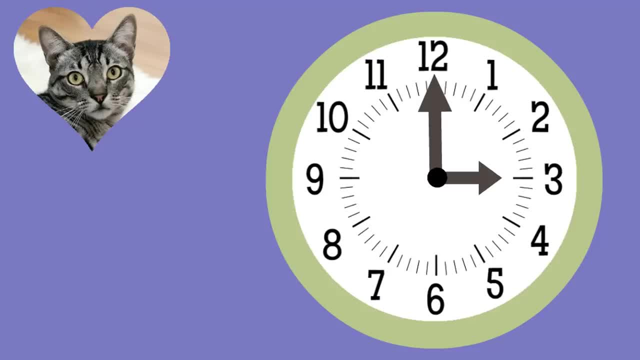 the trick. oh okay, so we need to count by fives to find out the minutes. that's a wonderful trick, that's amazing. you see, all of those little lines in between the numbers on the face of the clock represent one minute. to find out the minutes, we just have to count by fives around the clock, starting at the twelve. 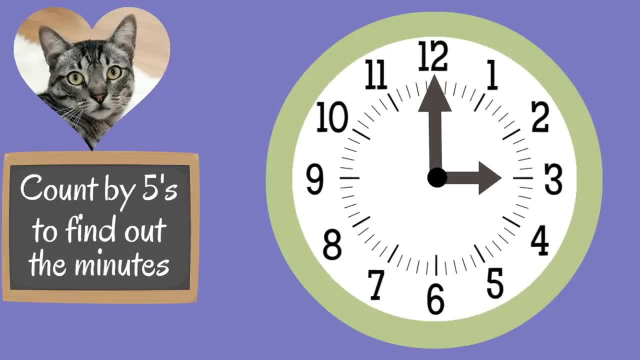 the twelve is like the starting line. when the minute is in the middle of the clock, When the minute hand is at the 12, that means zero minutes. Then the 1 is 5,, 2 is 10, then 15,, 20,, 25,, 30,, 35,, 40,, 45,, 50,, 55, and then back to zero. 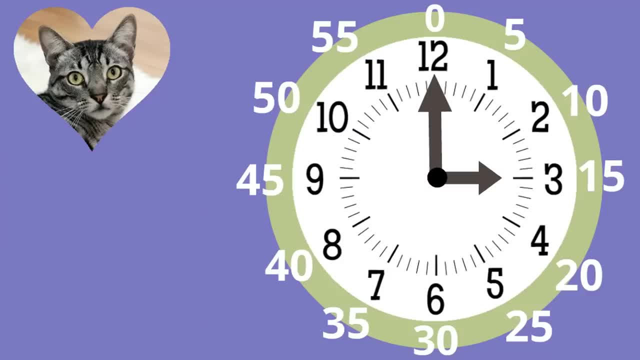 All we have to do is count by fives. Okay, so we're ready to figure out what time this is. Okay, so we already know what the hour is. The hour is 3.. Yes, Okay, so we write 3.. 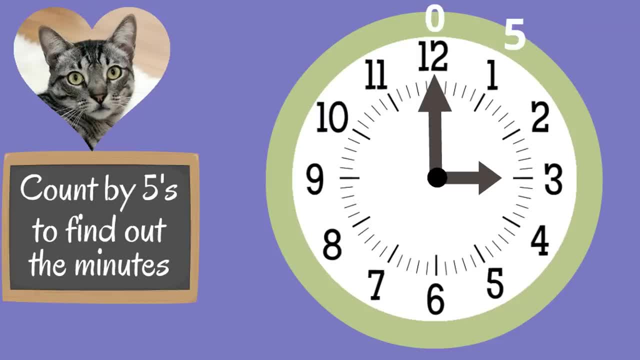 that means zero minutes. Then the one is five, two is 10, then 15,, 20,, 25,, 30,, 35,, 40,, 45,, 50,, 55, and then back to zero. All we have to do is count by fives. Okay, So we're ready to figure. 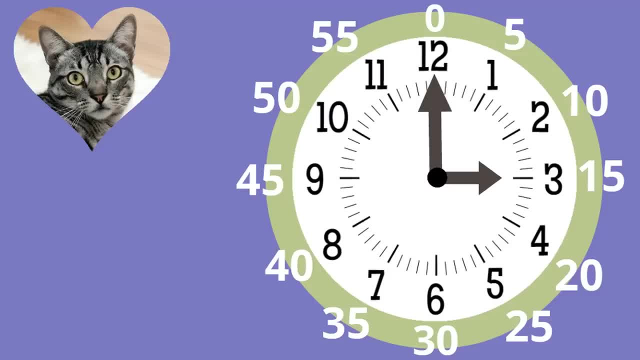 out what time. this is Okay, So we already know what the hour is. The hour is three, Yes, Okay, So we write three. Now we have to figure out the minutes, and the minute hand is pointing at the 12,. which means what? How many minutes? Zero, Yeah, And with minutes we always write two digits. 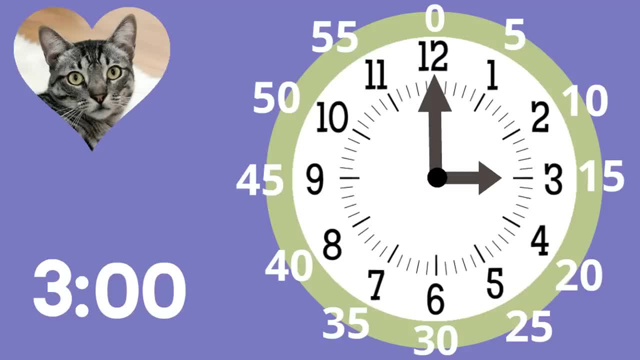 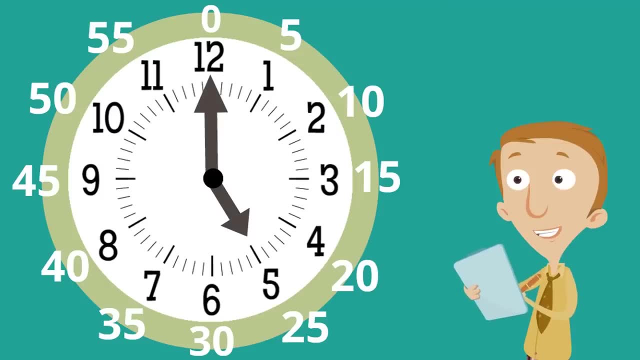 So we'll write two zeros. What is this time? Yeah, Great job. Okay, Let's try this one. What time does this clock say? Where's the hour hand? Yeah, On the five. And where's the minute hand? Yep, At the 12.. 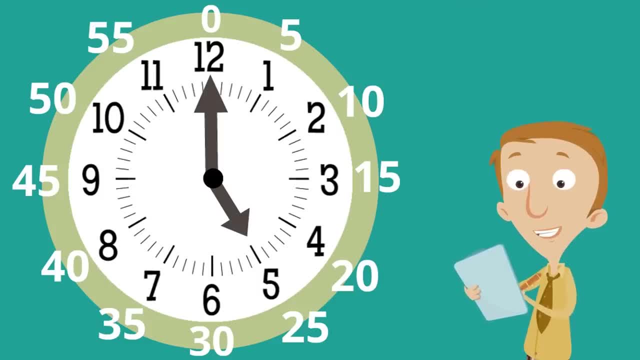 So you know there are zeros at the end of that. What time is it? Yes, It's five o'clock. Great job, All right, Let's try this one, Okay, Okay, Both hands are pointing at which number? Yeah, 12.. What time is this? 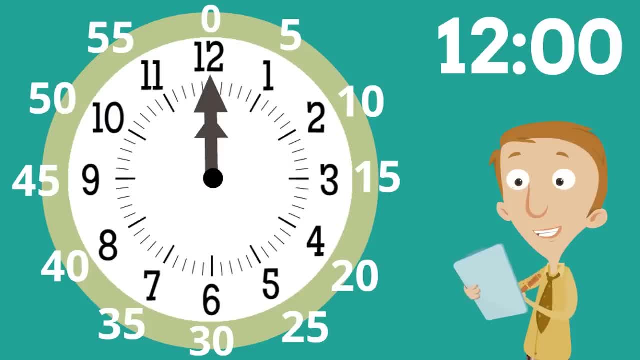 Yes, 12 o'clock, Great job. Notice, if the minute hand is pointing at the 12, you always say o'clock, So this is 12 o'clock. just like before we had three o'clock and five o'clock. This is 12 o'clock. 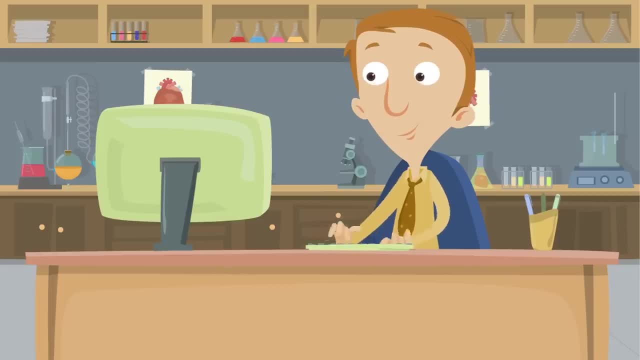 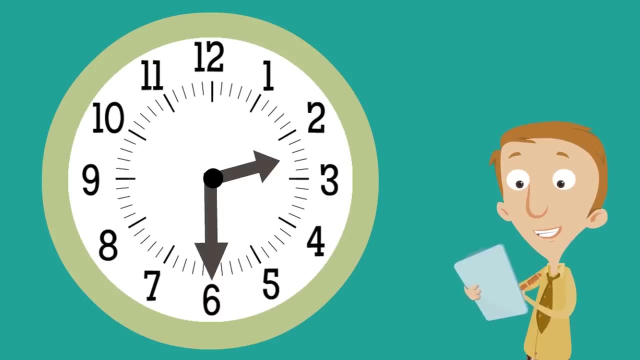 Terrific, We're going to change things up. Just remember our trick: Count by fives. Okay, Let's figure out what time this clock is showing us. First, let's look at the hour hand. Wait, It isn't directly pointing at a number, It is between the two and the three. 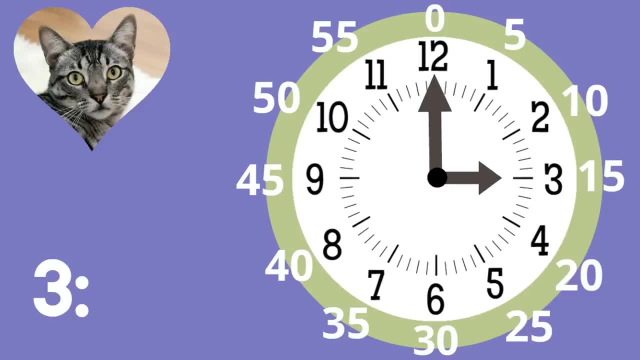 Now we have to figure out the minutes, and the minute hand is pointing at the 12, which means what? How many minutes? Zero, Yeah, and with minutes we always write two digits, so we'll write two zeros. What is this time? 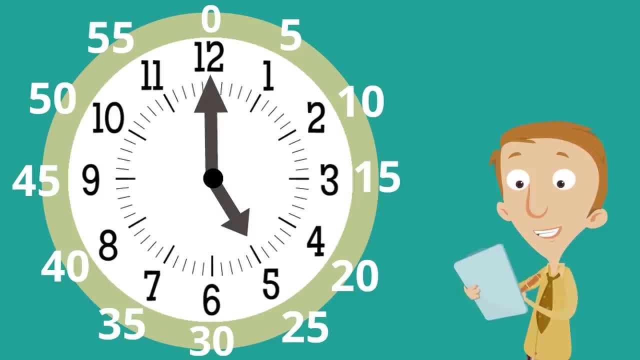 Yeah, 3 o'clock. Great, Good job. Okay, let's try this one. What time does this clock say? Where's the hour hand? Yeah, on the 5.. And where's the minute hand? Yep, at the 12.. 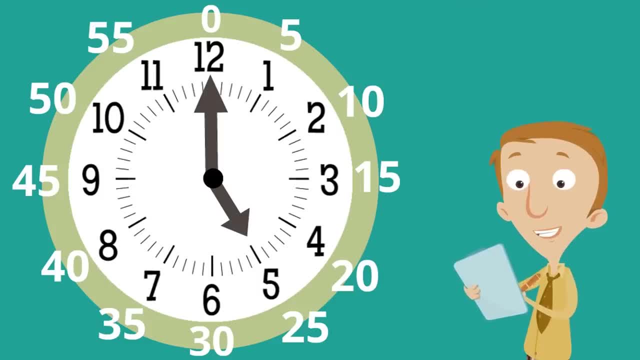 So you know there are zeros at the end of that. What time is it? Yes, it's 5 o'clock. Great job, All right, let's try this one. Okay, both hands are pointing at which number. Okay, both hands are pointing at which number. 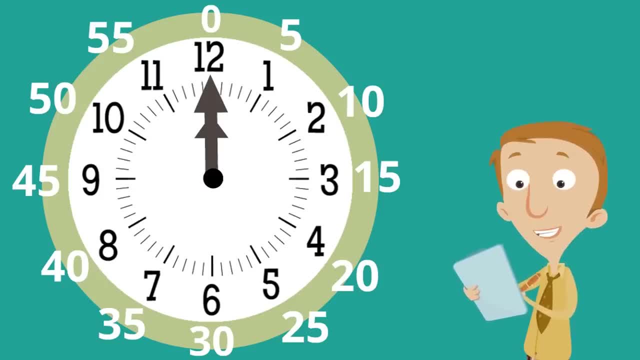 Yeah, 12.. What time is this? Yes, 12 o'clock, Great job. Notice, if the minute hand is pointing at the 12, you always say o'clock, So this is 12 o'clock, just like before we had 3 o'clock and 5 o'clock. 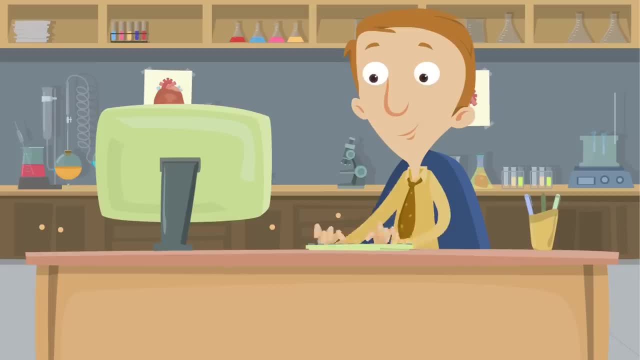 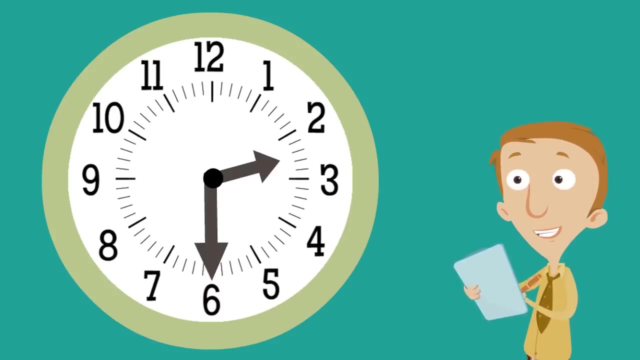 This is 12 o'clock. Terrific. Now we are going to change things up. Just remember our trick. our trick: count by fives. okay, Let's figure out what time this clock is showing us. First, let's look at the hour hand. Wait, it isn't directly pointing at a number. It is between the 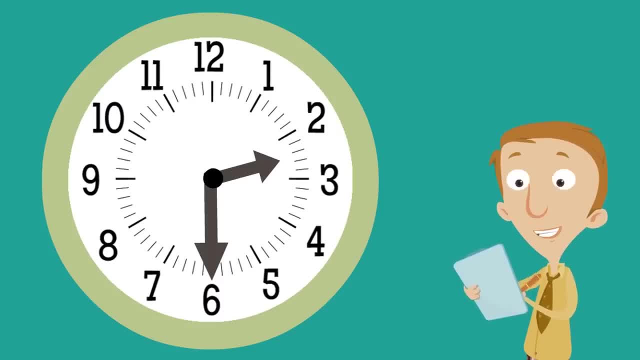 two and the three. No worries, When the hour hand is between two numbers, the hour is the earlier number, So the hour is two. Where is the minute hand pointing? That's right At the number six. we are going to use Mr Whisker's trick and count by fives. We start at the 12,, which is zero. 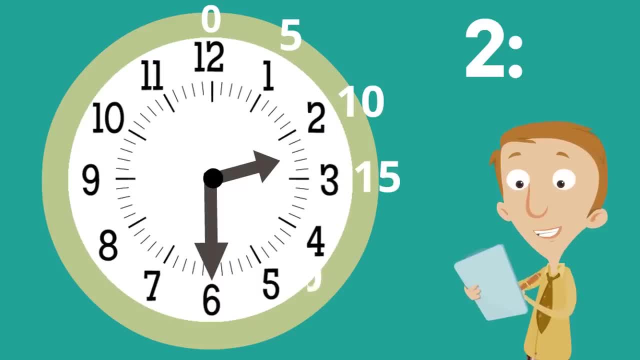 Then we count five, 10,, 15,, 20,, 25,, 30. So how many minutes is this showing? 30. That's right. So what time is the clock showing? 2.30.. You got it. 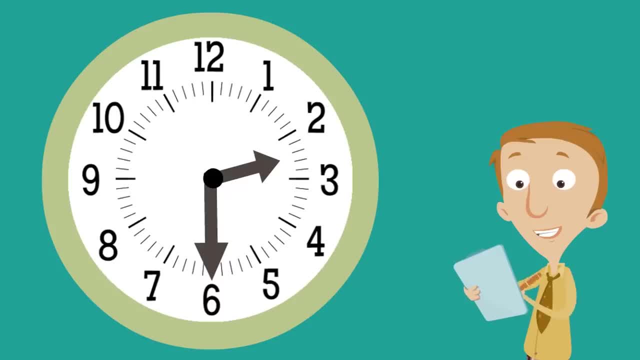 No worries, When the hour hand is between two numbers, the hour is the earlier number, So the hour is two. Where is the minute hand pointing? That's right At the number six. we are going to use Mr Whisker's trick and count by fives. We start at the 12,, which is zero, Then we count five, 10,, 15,, 20,, 25,, 30.. 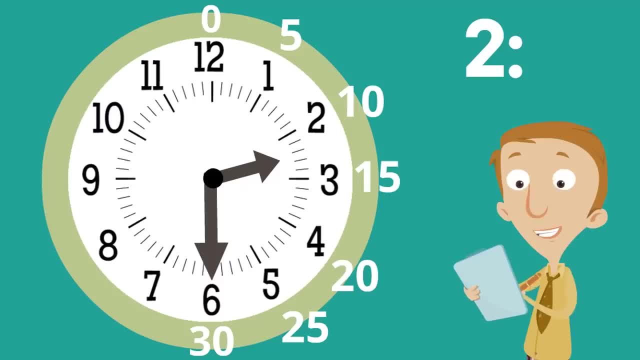 So how many minutes is this showing 30. That's right. So what time is the clock showing 2.30.. You got it. This one looks like fun. What time is it according to this clock? First let's look at the hour hand. The hour hand is between numbers. again, It is between which numbers. 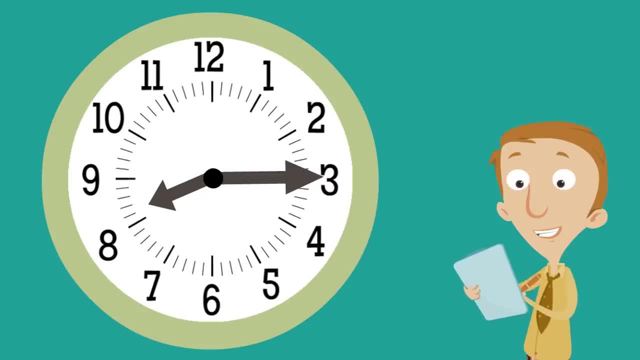 Yes, Eight and nine. Remember when the hour hand is between two numbers, the hour is the earlier number, So the hour is eight. Where is the minute hand pointing 30. That's right At the number three. we are going to use Mr Whisker's trick and count by fives. We start at the 12,, which is zero, Then we count five, 10,, 15.. So how many minutes is this showing? 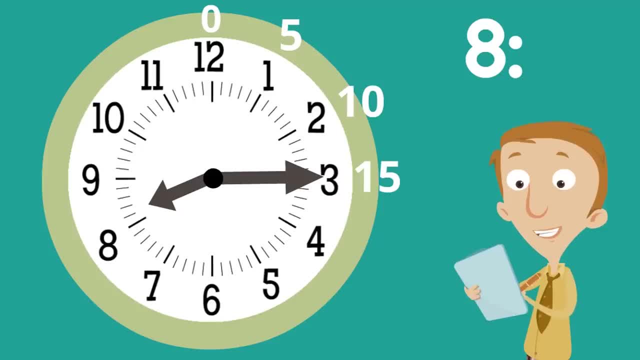 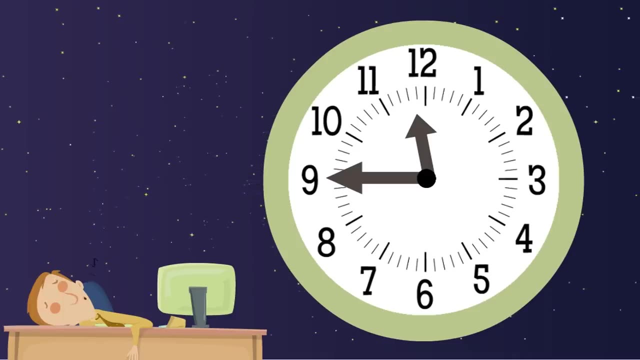 15.. Yeah, So what time is the clock showing? 8.15.. You got it. How about this one? What time is it according to this clock? First, let's look at the hour hand. The hour hand is between numbers. again, It is between which numbers? 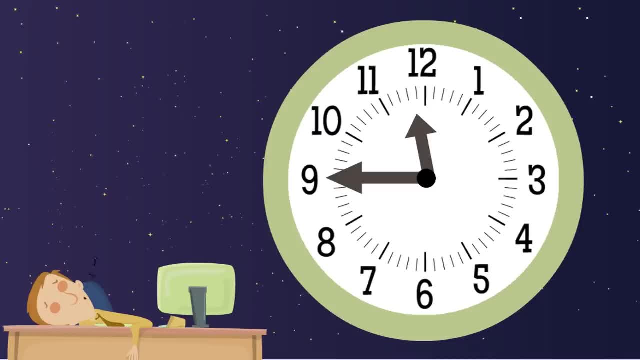 Yes, 11 and 12.. Remember, when the hour hand is between two numbers, the hour is the earlier number, So the hour is what? 11.. You are right, Okay, So where is the minute hand pointing? Yep, At the number nine. we are going to use Mr Whisker's trick and count by fives. We start with 12,, which is zero, Then we count five, 10,, 15,, 20,, 25,, 30,, 35,, 40,, 45. So how many minutes is this showing? 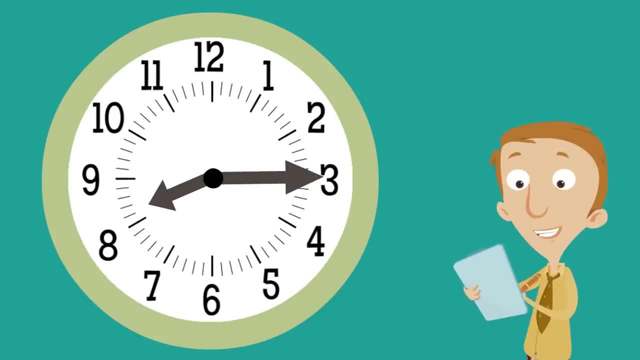 Okay, This is the hour hand pointing. We are going to use Mr Whisker's trick and count by fives. This one looks like fun. What time is it according to this clock? First, let's look at the hour hand. 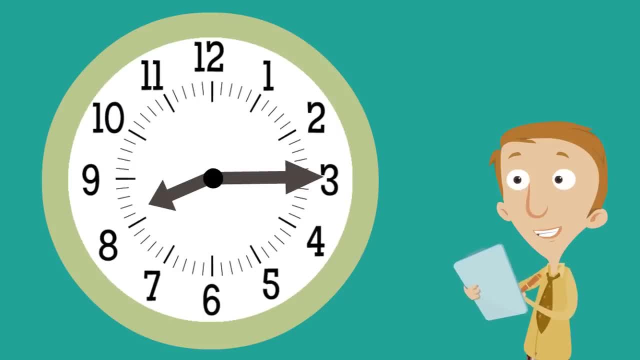 The hour hand is between numbers. again, It is between which numbers? Yes, eight and nine. Remember, when the hour hand is between two numbers, the hour is the earlier number, So the hour is eight. Where is the minute hand pointing? That's right. 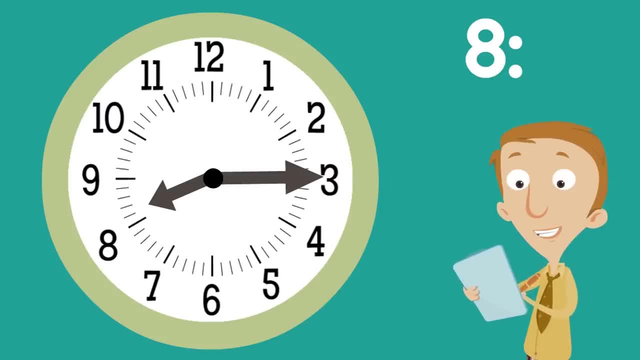 At the number three. we are going to use Mr Whisker's trick and count by fives. We start at the 12,, which is zero, Then we count five, 10,, 15.. So how many minutes is this showing? 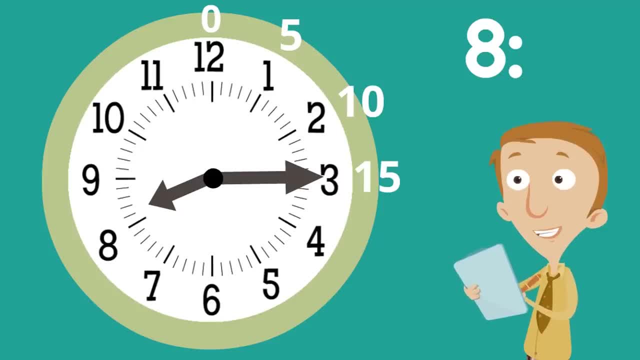 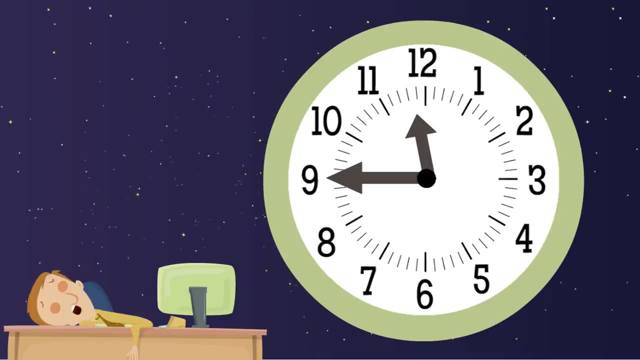 15.. Yeah, So what time is the clock showing? 8.15.. You got it, Okay. How about this one? What time is it according to this clock? First, let's look at the hour hand. The hour hand is between numbers. again, It is between which numbers? 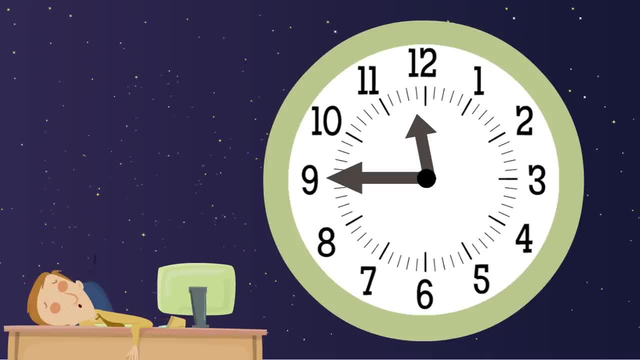 Yes, 11 and 12.. Remember, when the hour hand is between two numbers, the hour is the earlier number. So the hour is what? 11. 11. You are right, Okay, So where is the minute hand pointing? 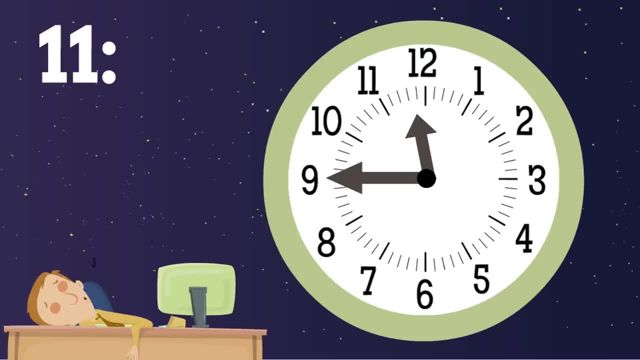 Yep At the number nine. we are going to use Mr Whisker's trick and count by fives. We start with 12,, which is zero, Then we count five, 10,, 15,, 20,, 25,, 30,, 35,, 40,, 45. So how many minutes is? 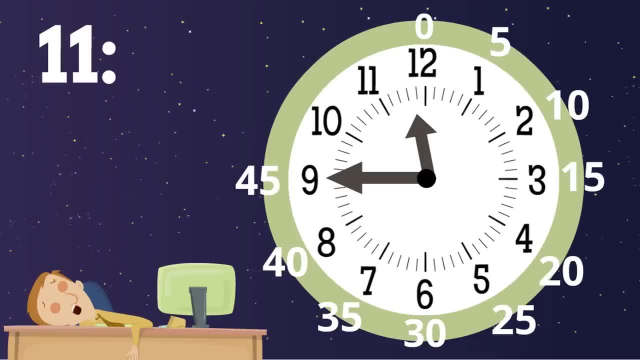 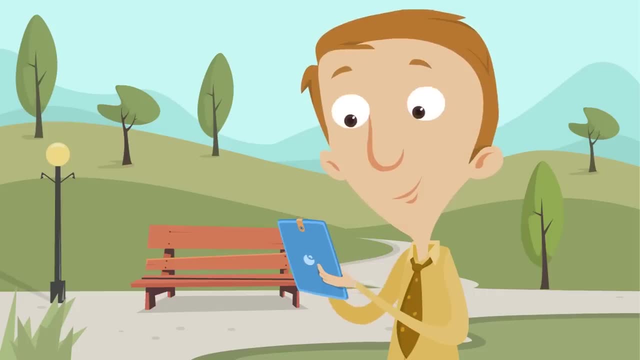 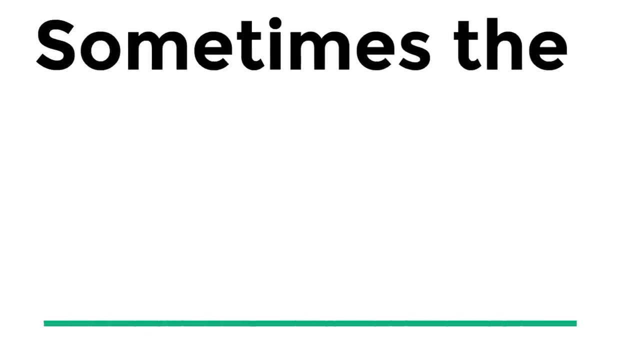 this showing 45.. You got it, So what time is this clock showing? 11.45.. Yes, Great job. We looked at examples of when the hour hand isn't pointing directly at a number on the face of a clock. You know, sometimes the minute hand isn't pointing directly at a number. 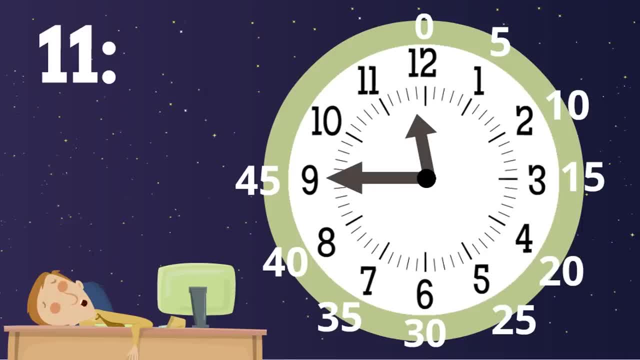 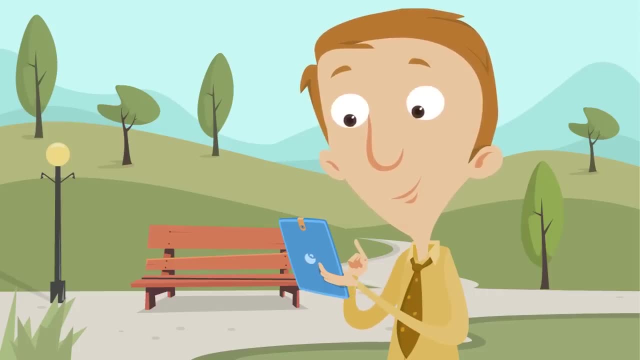 45.. You got it, So what time is the clock showing? 11.45.. Yes, Great job. We looked at examples of when the hour hand isn't pointing directly at a number on the face of a clock. You know, sometimes the minute hand isn't pointing directly at a number. 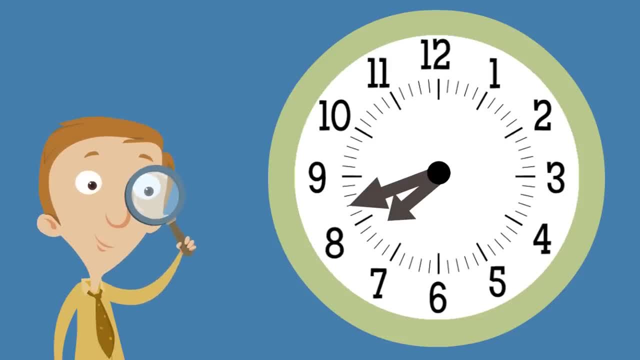 Look at this example. The hour hand is between which two numbers? Yes, Seven and eight. Which number is the hour? Yep, Seven. The hour is always the earlier number on the clock when it is between two numbers. Now the minute hand is near the eight, but notice, it went past the eight by two. To figure out the minutes, we will count by fives, just like before, and then add two at the end. 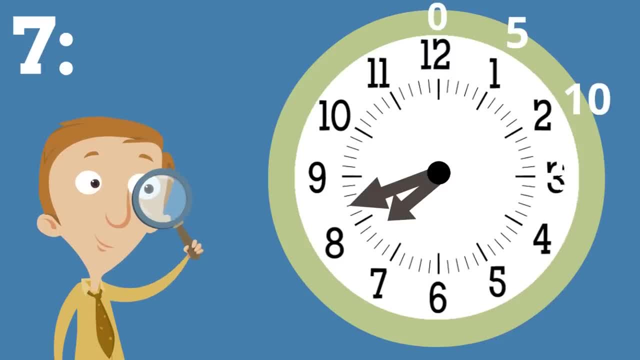 The 12 is zero five, 10.. 15,, 20,, 25,, 30,, 35,, 40. Then you just add 40 plus two. You got to add two. What is 40 plus two? 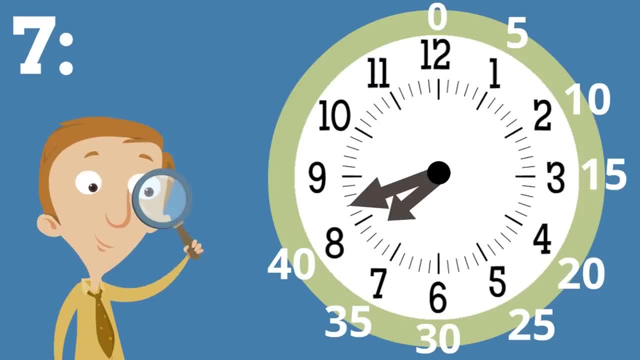 Yeah, 42. So the time is 742.. Wonderful job, That's great. Let's look at one last analog clock. Just looking at this clock, what is the hour? Yes, 12, because 12 is the earlier hour on the clock. 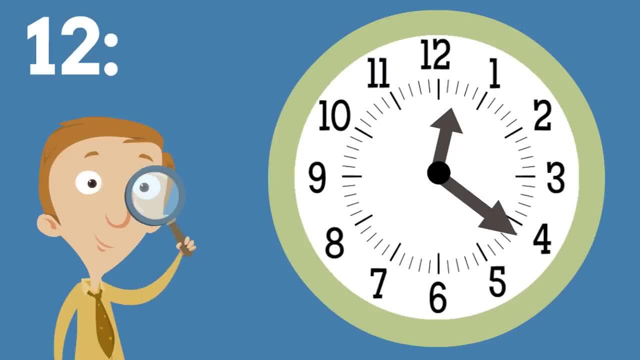 How about the minutes? Use the count by fives trick and notice the minute hand is one minute after the four. You'll need to add one minute, All right, 21.. So the time is 1221.. Let's check the minutes to be sure. 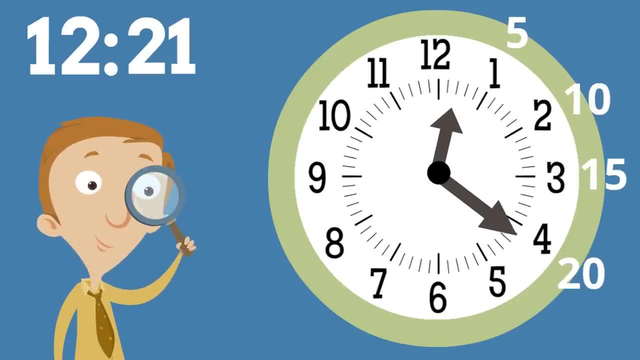 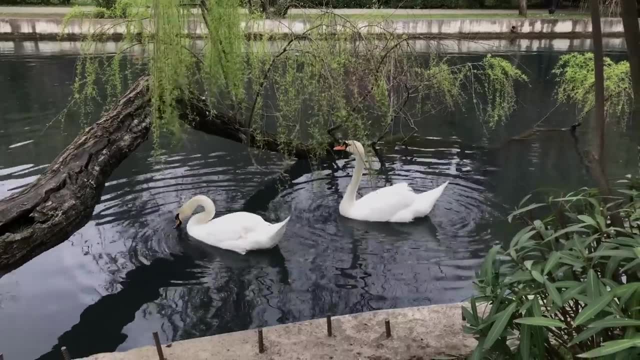 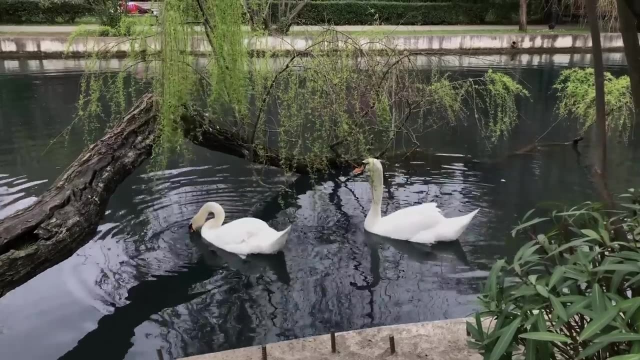 Five, 10,, 15,, 20, then add one which is 21.. You have done a great job. Before we conclude this video, we want to share two more things. What's with the swans? We are sharing two things about analog clocks. 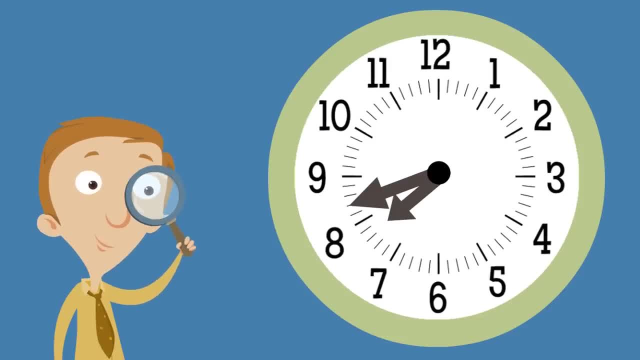 Look at this example. The hour hand is between which two numbers? Yes, Seven and eight. Which number is the hour? Yep, Seven. The hour is always the earlier number on the clock when it is between two numbers. Now the minute hand is near the eight, but notice it went past the eight by two To figure out the 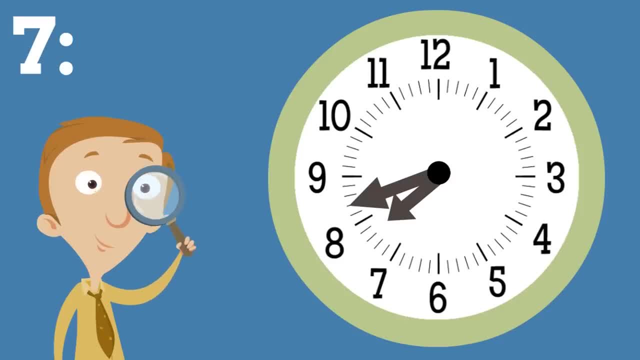 minutes. we will count by fives, just like before, and then add two at the end. The 12 is zero. The minute hand is, after 12, 15100.. The time being, 410 is equal to 1270.. So you have to. 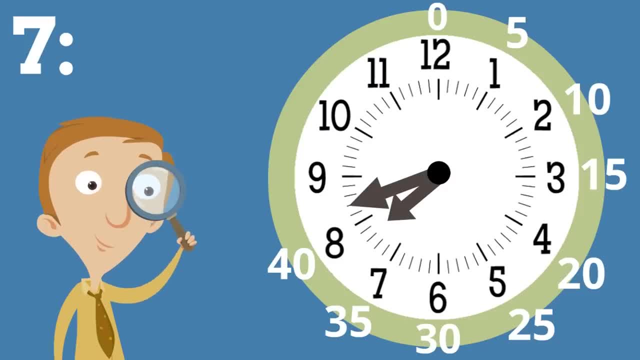 keep counting: 10,5,0, 5,10,, 15,20,, 25,30, 35,40.. Then you just add 40 plus 2.. You got to add two. What is 40 plus 2?? Yeah, 42.. So the time is 7.42.. Wonderful. 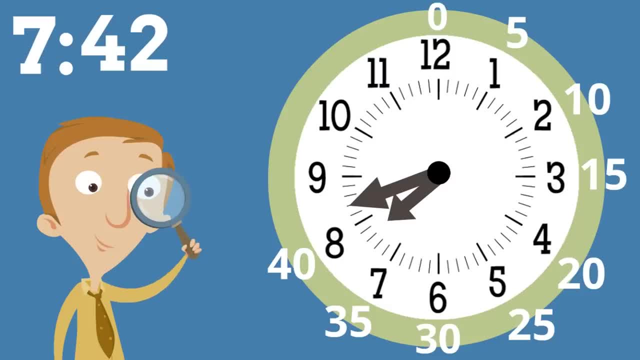 job. that's great. Let's look at one last analog clock. Just look, uh, at all the different analog clocks. Let's just focus on what is just the time. so what's the multiple you're guessin'? Can you see those numbers if you mess up? 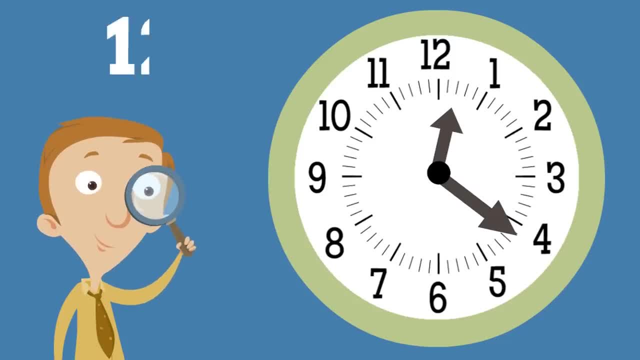 looking at this clock, what is the hour? Yes, 12, because 12 is the earlier hour on the clock. How about the minutes? Use the count by fives. trick and notice the minute hand is one minute after the four. You'll need to add one minute. 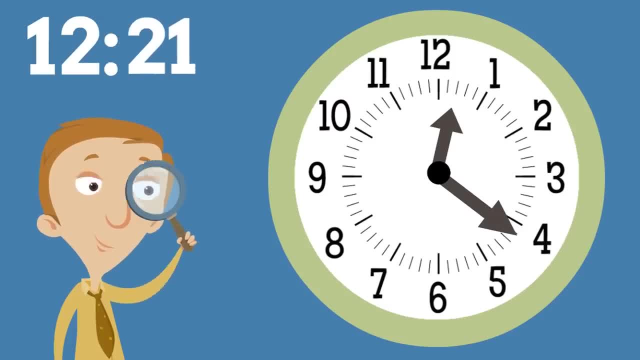 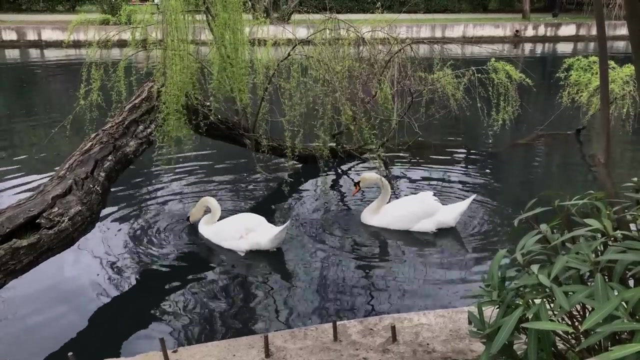 All right, 21.. So the time is 1221.. Let's check the minutes to be sure: Five, 10,, 15,, 20, then add one which is 21.. You have done a great job. Before we conclude this video, we want to share two more things. What's with the swans? We are. 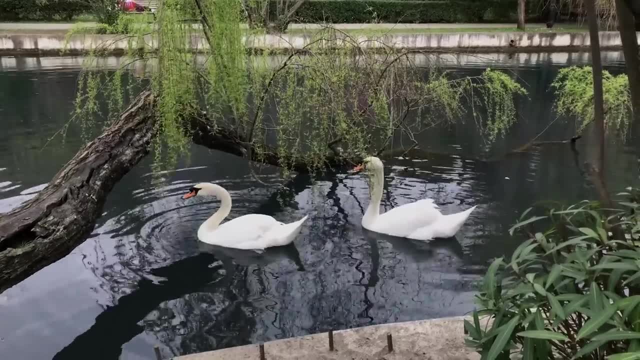 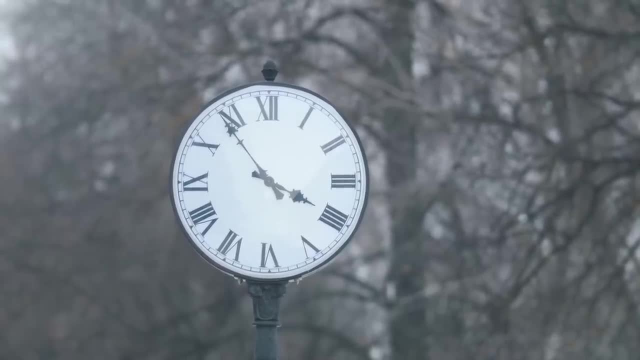 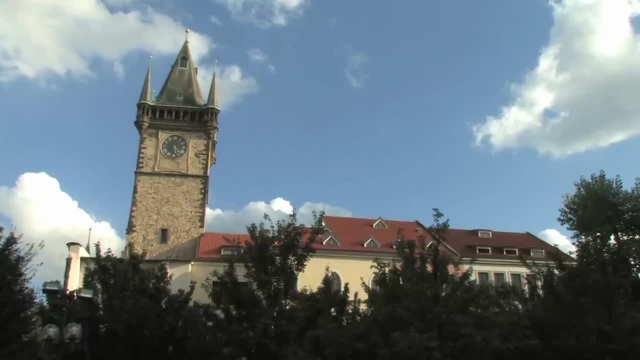 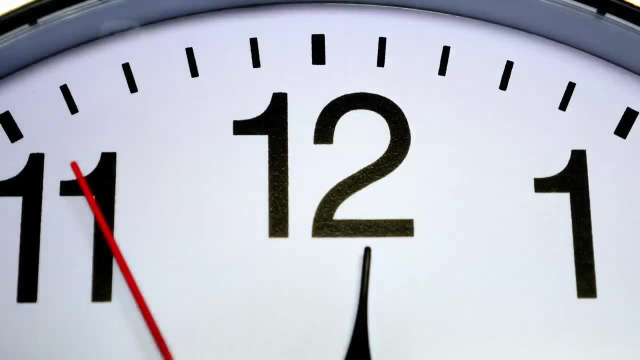 regular numbers. Fancy clocks and clock towers usually use Roman numerals. If you need help with Roman numerals, we do have a video about that. The second thing is that you may see a thin hand, sometimes a different color than the hour and minute hands. that shows the seconds.